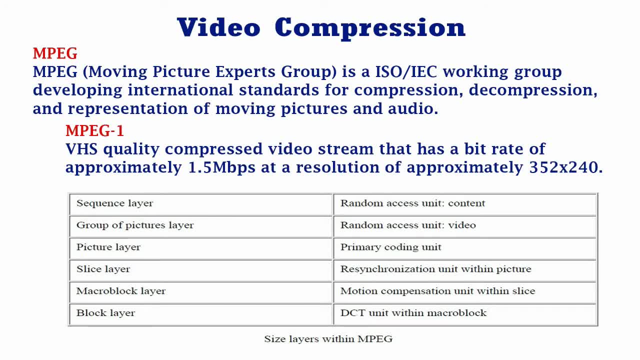 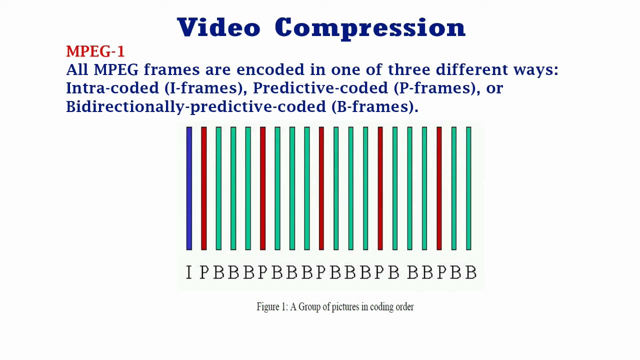 that provide the ability to randomly access a video sequence, as well as provide a barrier against corrupted information. Size layers within MPEG are given in table. All MPEG frames are encoded in one of three different ways: Intra-coded, Predictive-coded or Bidirectionally Predictive-coded. 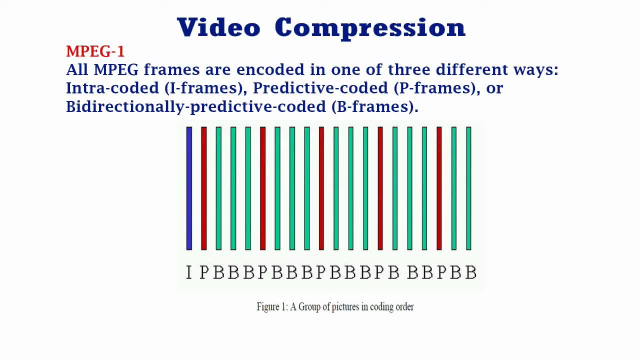 I-frames are encoded in two ways. I-frames are encoded as discrete frames, independent of adjacent frames. Thus they provide randomly accessible point within the video stream. Because of this, I-frames have the worst compression ratio of the three other frames. 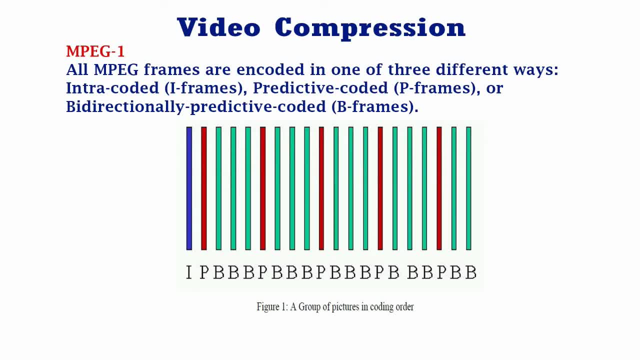 P-frames are coded with respect to a past I-frame or P-frame, resulting in smaller encoded frame size than the I-frames. The B-frames require a preceding and future frame, which may be either I-frames or P-frames, in order to be decoded. 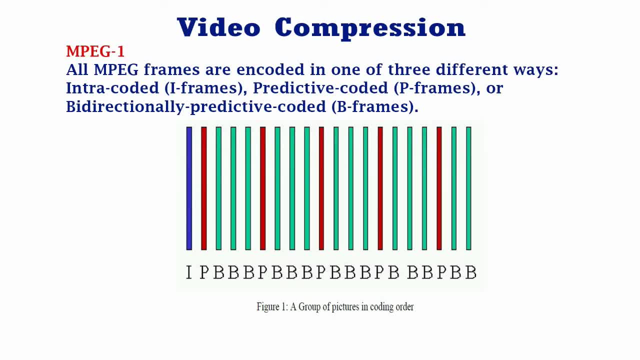 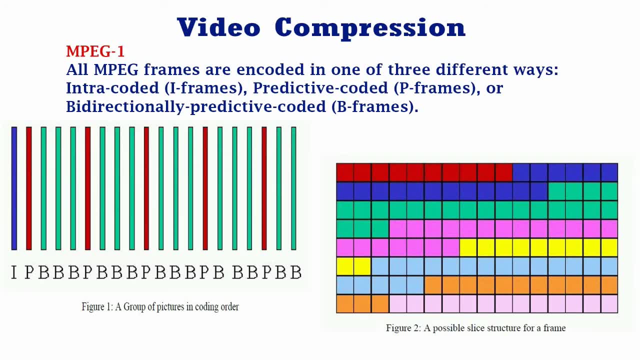 But they offer a highest degree of compression. As can be seen in table, an MPEG video consists of many video sequences, Each of which has many groups of pictures in it. Typically, a group of pictures, that is GOP, has a single I-frame and many P- and B-frames. 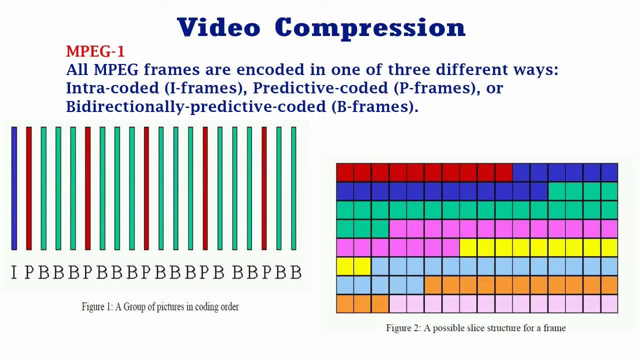 Although there is no limit on the size of GOP and values around 15 is common, The total GOP is given in figure 1.. The frames are divided in a block size of 16 by 16 and these blocks are called macro blocks. A sequence of macro blocks is called a slice. 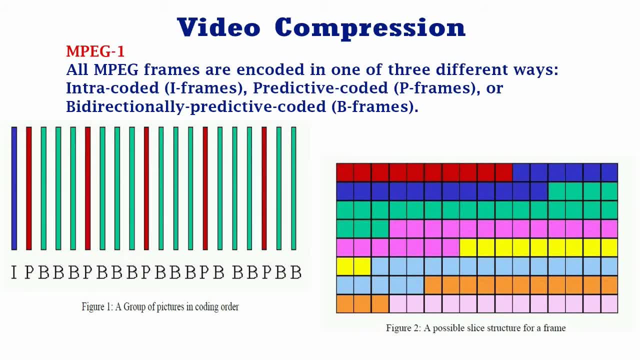 A slice can be an entire row of macro blocks or it can start in one row and end in another. Each frame consists of many slices. A possible slice structure is given in figure 2.. Each color represents a different slice. Most of the parameters can be specified during the encoding stage. 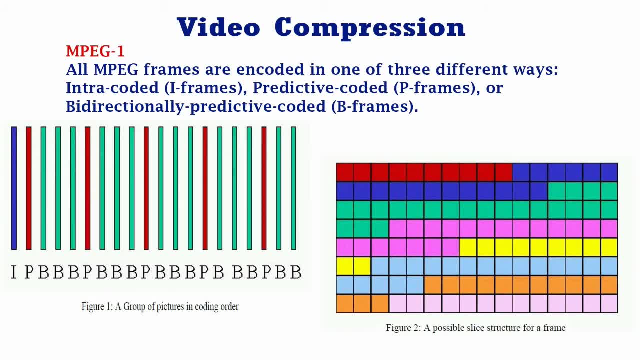 You can specify the GOP pattern, size of slice, desired number of frames per second, etc. Each of these layers has a header used for synchronization. If part of a slice is lost, the decoder will skip the rest of the slice when it detects the error. 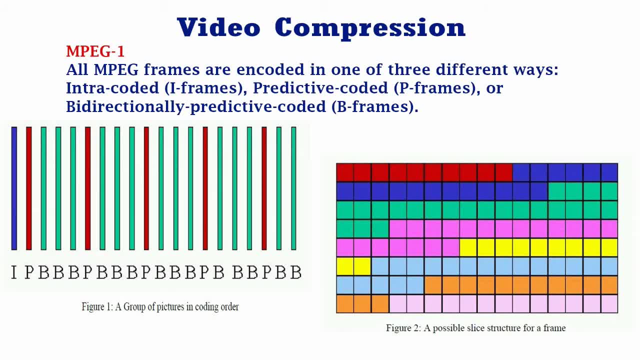 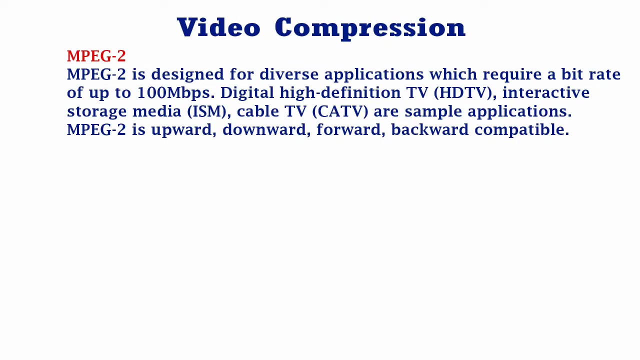 and start decoding from the beginning of the next slice. Video decoding is a computationally expensive operation. MPEG-1 decoding can be done in real time using a 350 MHz Pentium processor. MPEG-2 MPEG-1 has a bitrate of about 1.5 Mbps. 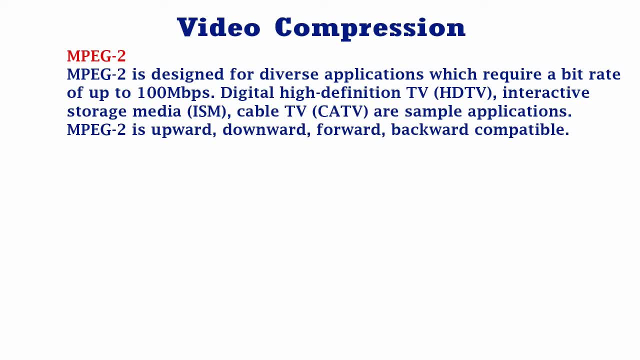 MPEG-2 is designed for diverse applications which require a bitrate of up to 100 Mbps. Digital High Definition TV, Interactive Storage Media, Cable TV are sample applications. Multiple video formats can be used in MPEG-2 coding to support these diverse applications. 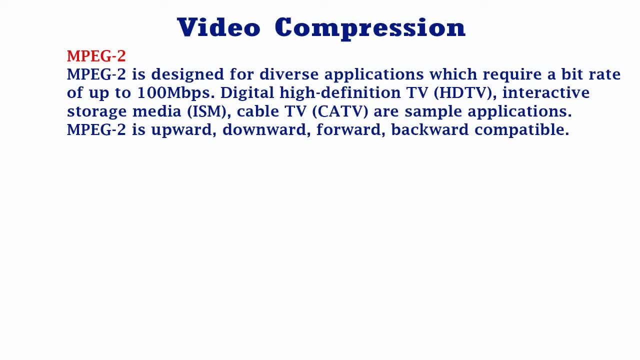 MPEG-2 has bitstream scalability and it is possible to extract a lower bitstream to get lower resolution or frame rate. Decoding MPEG-2 is a costly process. Bitstream scalability allows flexibility in the required processing power for decoding MPEG-2 is upward. 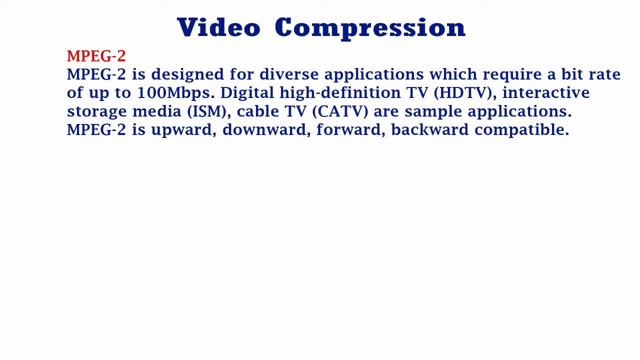 downward, forward, backward compatible. Upward compatibility means the decoder can decode the pictures generated by a lower resolution encoder. Downward compatibility implies that a decoder can decode the picture generated by a higher resolution encoder. In forward compatible system, a new generation decoder can decode the pictures. 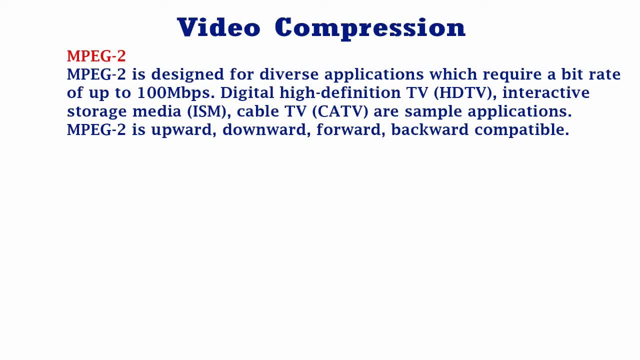 generated by an existing encoder And in a backward compatible system, existing decoder can decode the pictures generated by new encoder. In MPEG-2, the input data is interlaced, since it is more oriented towards television applications, Video sequence layers are similar to MPEG-1. 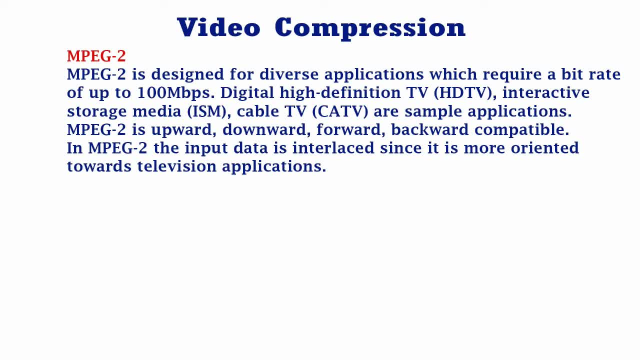 The only improvements are field or frame motion compensation and DCT processing, as well as scalability. Macro blocks in MPEG-2 has two additional chrominance blocks. when 4x2x2 input format is used, 8x8 block size is retained in MPEG-2. 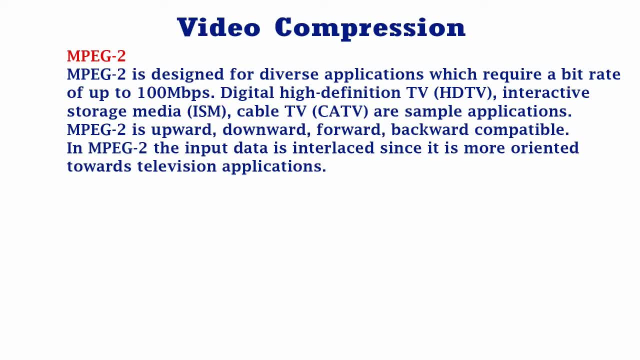 In scaled format, blocks can be 1x1,, 2x2, 4x4. for resolution enhancement, P and B frames have frame and field motion vectors. MPEG-2 decoding cannot be done in real time with current processors. MPEG-3. 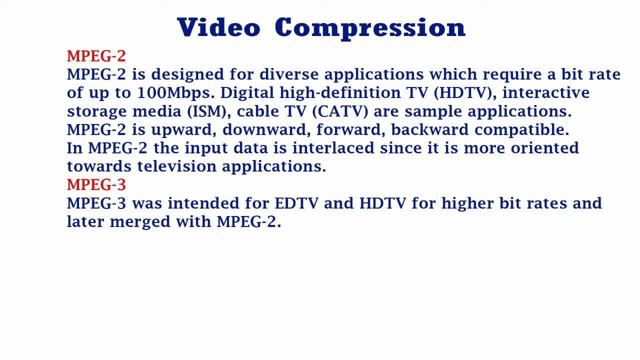 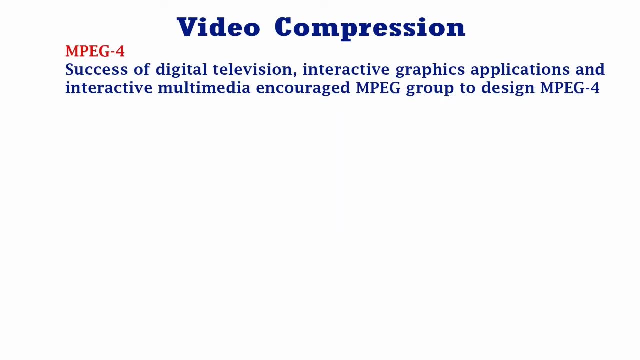 MPEG-3 was intended for EDTV and HDTV for higher bit rates, and latter merged with MPEG-2. MPEG-4 Success of digital television, interactive graphic applications and interactive multimedia encouraged MPEG group to design MPEG-4.. MPEG-4 allows the user to interact with the objects. 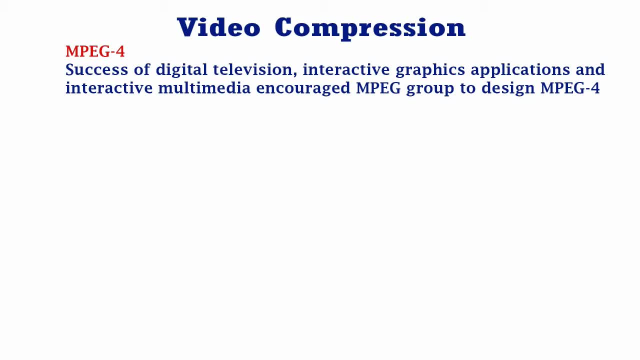 in the scene within the limits set by the author. It also brings multimedia to low bitrate networks. MPEG-4 uses media objects to represent oral, visual or audiovisual content. Media objects can be synthetic, like interactive graphics applications, or natural, like in digital television. 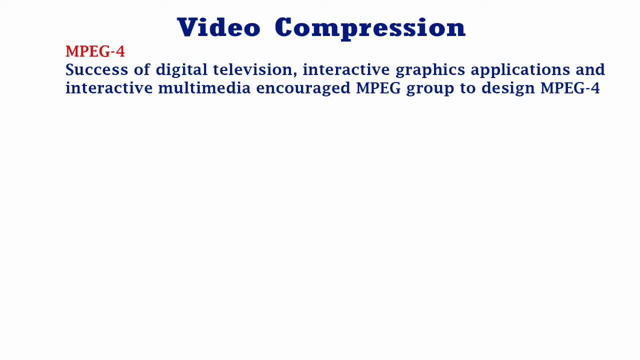 These media objects can be combined to form compound media objects. MPEG-4 multiplexes and synchronizes the media objects before transmission to provide quality of service, and it allows interaction with the constructed scenes at receiver's machine. MPEG-4 organizes the media objects in a hierarchical fashion. 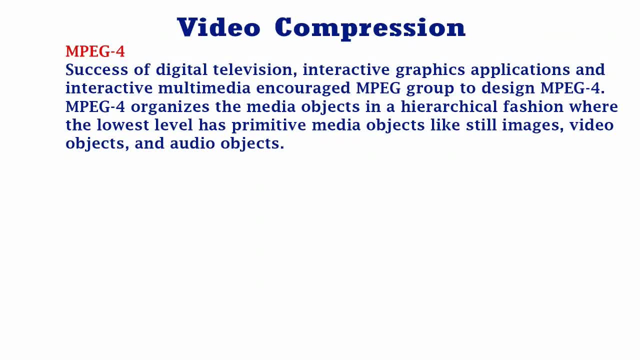 where the lowest level, as primitive media objects like still images, video objects and audio objects. MPEG-4 has a number of primitive media objects which can be used to represent two or three-dimensional media objects. MPEG-4 also defines a coded representation of objects. 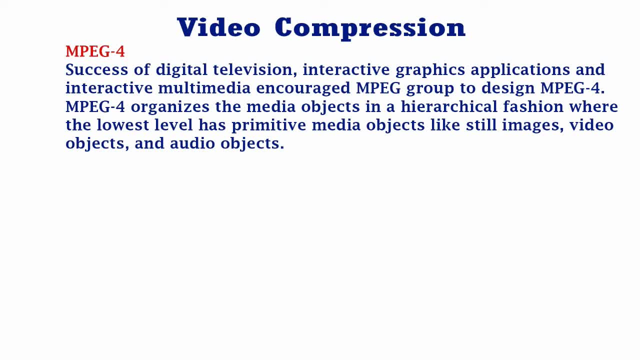 for text, graphics, synthetic sound, audio and video. MPEG-4 provides a standardized way to describe a scene. Media objects can be placed anywhere in the coordinate system. Transformations can be used to change the geometric or acoustical appearance of a media object. 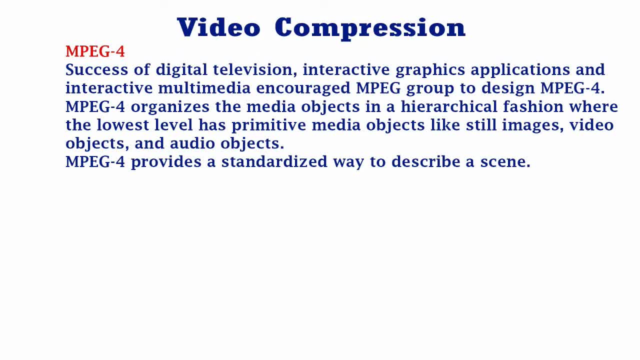 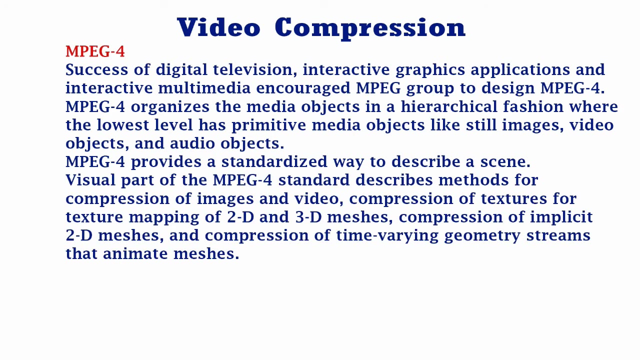 Primitive media objects can be grouped to form compound media objects. Streamed data can be applied to media objects to modify their attributes and the user's viewing or listening points can be changed to anywhere in the scene. Visual part of the MPEG-4 standard describes the method. 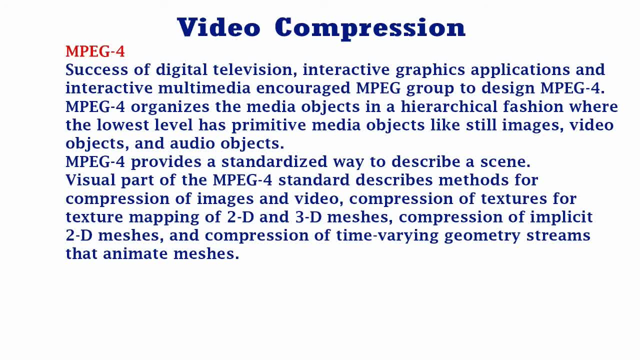 for compression of images and video, Compression of textures, for texture mapping of 2D and 3D meshes, Compression of implicit 2D meshes and compression of time-varying geometry streams that animate meshes. It also provides the algorithms for random access. 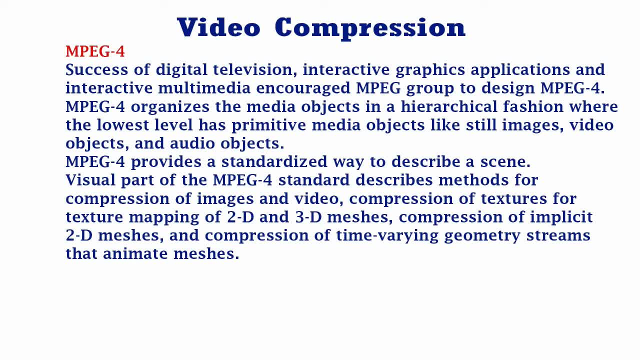 to all types of visual objects, as well as algorithms for spatial, temporal and quality scalability, content-based scalability of textures, images and video. Algorithms for error robustness and resilience in error-prone environments are also part of the standard For synthetic objects. 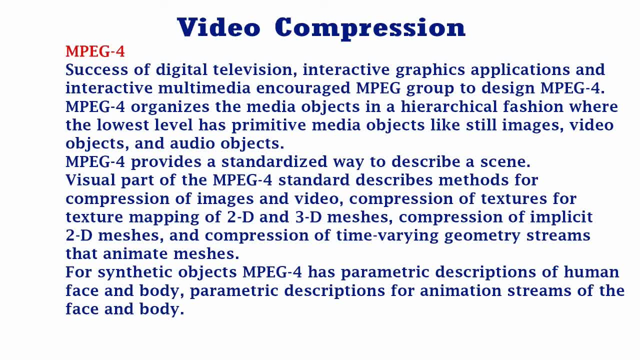 MPEG-4 has a parametric description of human face and body, Parametric description for animation streams of the face and body. MPEG-4 also describes static and dynamic mesh coding with texture mapping, texture coding with view-dependent applications. MPEG-4 supports coding of video. 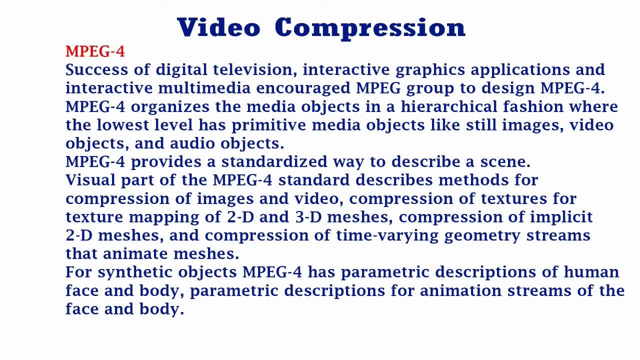 with spatial and temporal scalability. Scalability allows decoding a part of a stream and construct images with reduced decoder complexity, reduced spatial resolution, reduced temporal resolution, or with equal temporal and spatial resolution or reduced quality. Scalability is desired when video is sent over heterogeneous network. 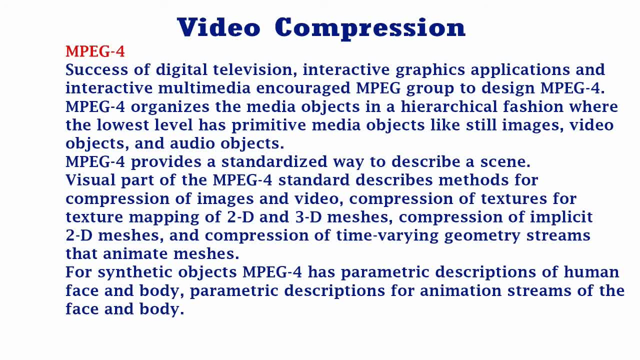 or receiver cannot display at full resolution, that is, with limited power. Robustness in error-prone environment is an important issue for mobile communications. MPEG-4 has three groups. It has three groups of tools for this. A resynchronization tool enables the resynchronization.